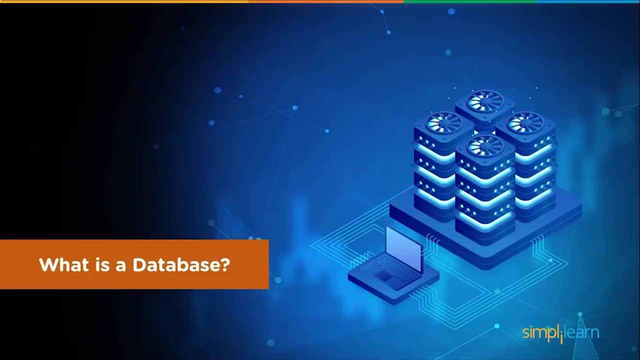 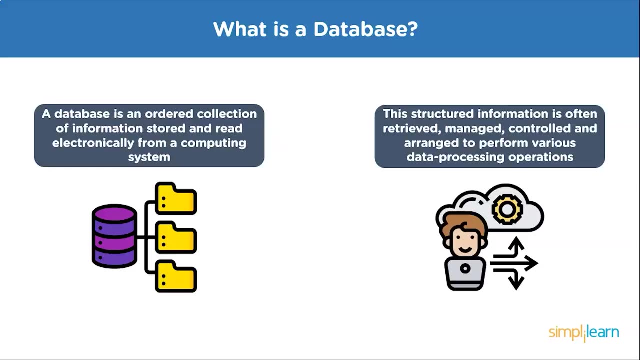 management system. If we talk about database, it is an ordered collection of information stored and read electronically from a computing system, For example Flipkart. Flipkart stores data of its customers when they log into their account After search for their browsing history. this old data is stored at a server as a database. 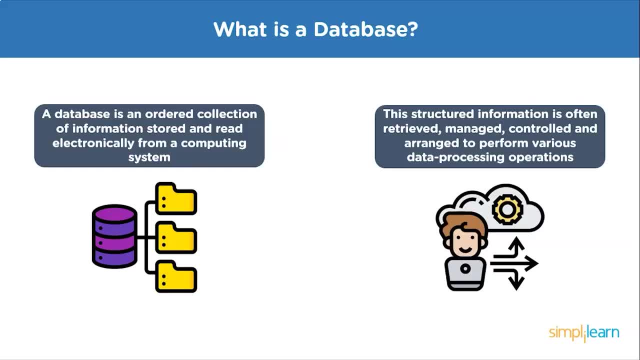 And further. database is also of two types: Structured database and unstructured database. Structured database is where we can store data in a particular structure, whereas for unstructured data, there is no particular structure to store data, For example, webpage. 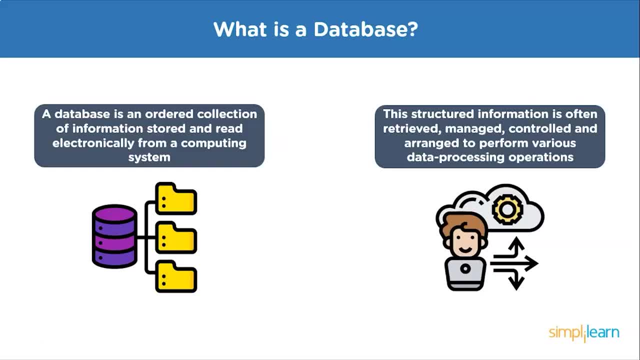 which is a collection of images, videos, text, which has no particular format, is a form of unstructured database. In fact, today we are going to learn how to store data in a structured database. Let's see what is unstructured database. 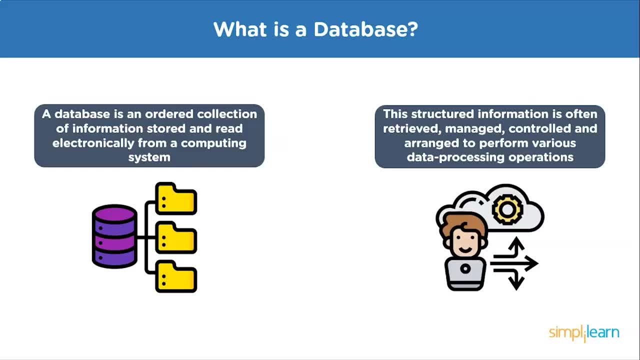 Structured database is where 90% of the data on the planet is unstructured, Whereas structured database is stored in a particular structure, that is, tables, And the best example for structured databases is relational database system, or DBMS, which stores data in a form. 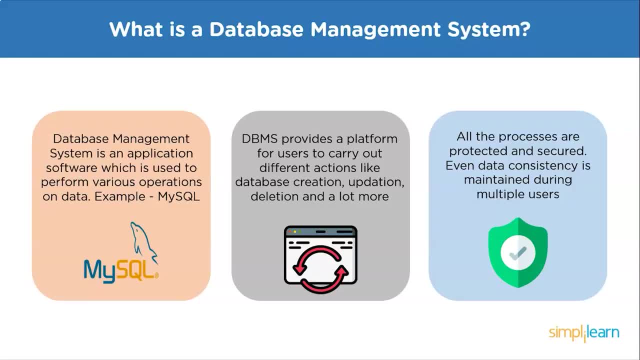 of relations, that is, tables, And if a user want to access the data or want to perform some operations on the data. DBMS is the entity which allows users to perform different operations on data And to perform these operations we are required to have a database with a specific structure that 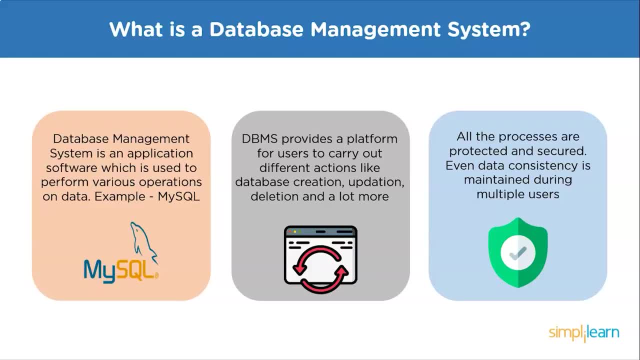 available with different versions of database management systems like MySQL, SQLite, PostgreSQL and Oracle Database. So now we will see what advantages DBMS has, through which it has replaced the flat file system. It doesn't mean that the flat file system is not used. now Let's see a scenario In the 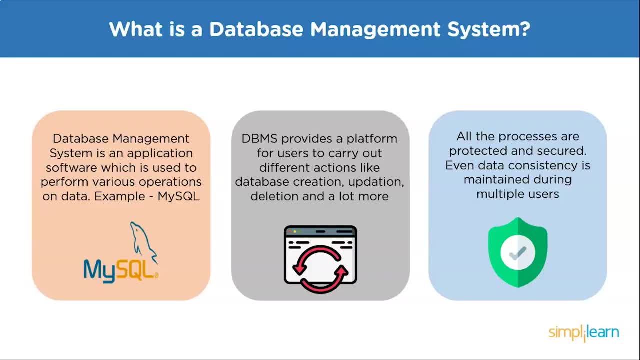 1970s, the data was stored in flat file system and can be accessed there only. Like in our laptops, we also get a flat file system which is inbuilt to be operated by operating systems with drives like CIFS, NFS, and in these drives 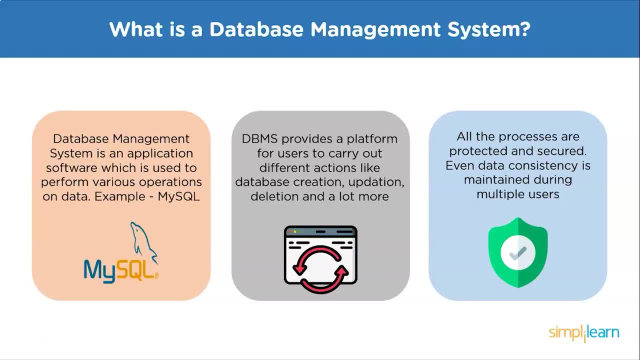 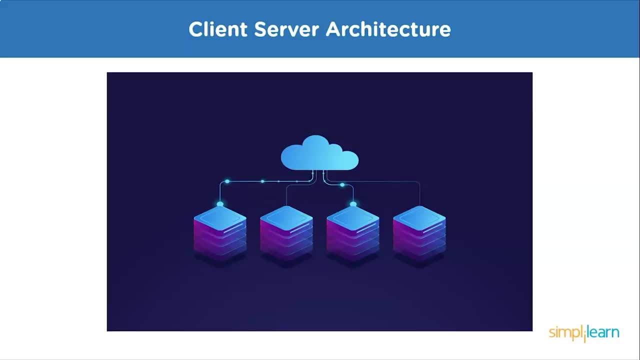 data is stored in the hierarchical form. So what was the need for DBMS? In today's time, we use client-server architecture. Due to this architecture, not only you have access to your data, but if you want to give access to different persons on the planet, you can. Now we will just have a. 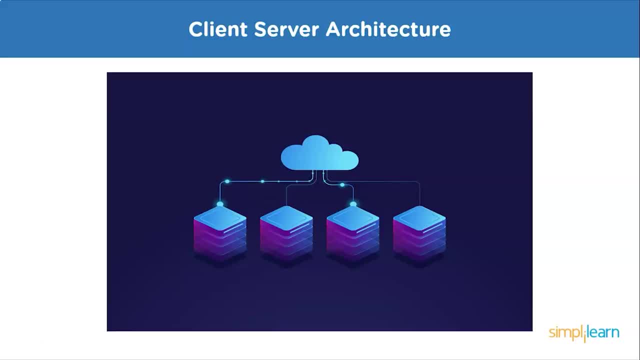 look at what client server architecture is. In client server architecture, the data is stored in a centralized location and the users from across the world can access the data Here. flat file systems can't be used to fulfill this purpose. We have to use DBMS. The reason being is when we search for data, for example a 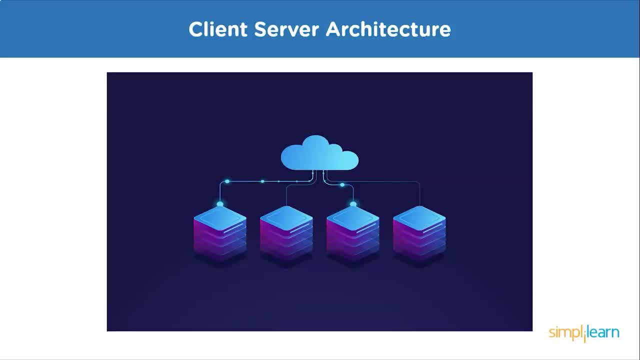 particular product on Flipkart, it will show the results in seconds. but if we have to search the same product in flat file system we have around fifteen GB of data of products and when we use DBMS it has stored the 50 GB data at Flipkart server. now user will just write a simple query through SQL and get the 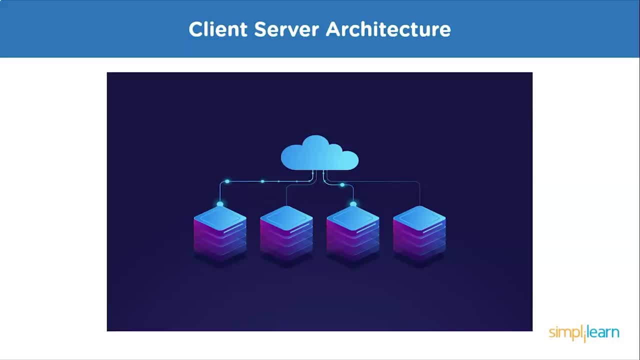 data about the particular product. searching is fast and memory utilization is efficient. and not only this: when we have to search for a file in flat file system, we should know the attributes of file, like its location name, with the metadata metadata, it's the data about the data that is data about. 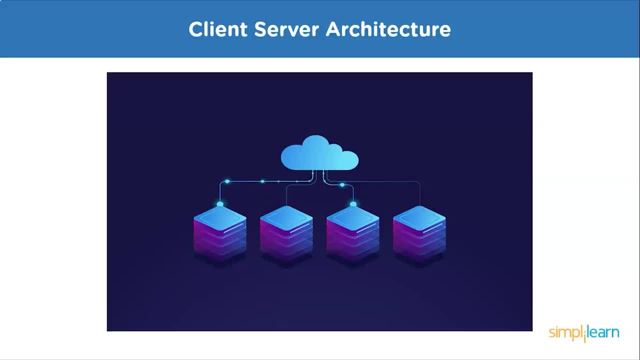 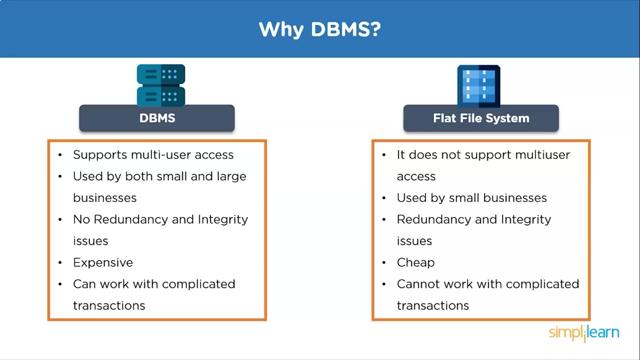 particular file. but in DBMS, user does not know where data is stored. we just send a request and the request is sent to server and we can access the data. now we will see why DBMS and the first thing we will see is concurrency: multiple people access the data at same time, for example, when you are accessing the 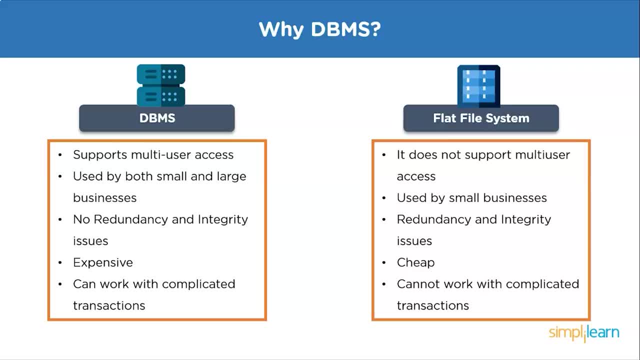 application of Flipkart, there are multiple users who are accessing the application and searching for the same product. if it was based on flat file system, it won't be possible. DBMS has protocols for concurrency security security, also known as role based security. if we have data and to 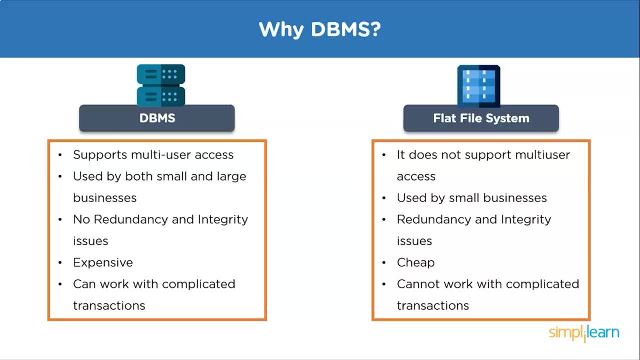 access their data. different users have different access. this is role based access control, whereas flat file system is operated by operating system which has no role based security protocol and particular data is visible. data residency: it means duplicacy in file system. we can store same content with different file names. 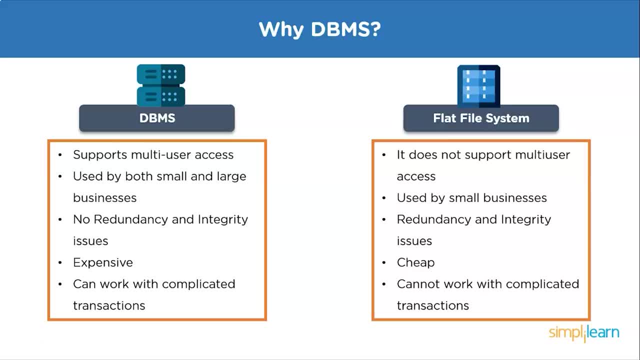 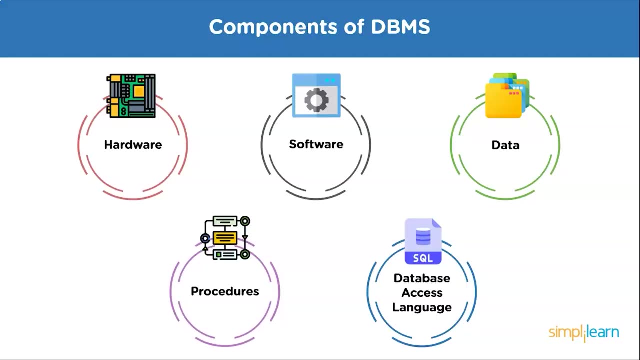 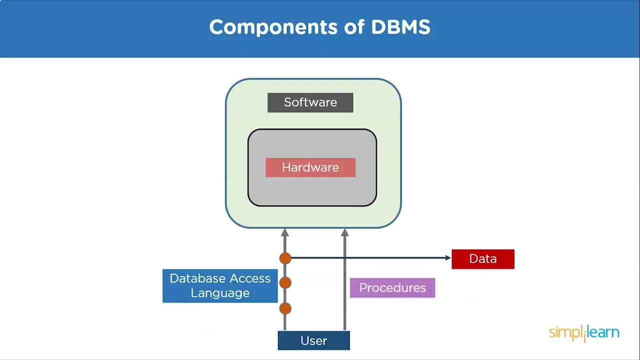 in flat file system, whereas DBMS has protocols and keys to tackle these problems. that's why DBMS is used for client-server architecture. now we will see the components of DBMS: hardware, software, data procedures and database access language. let's have a simple diagram to see how all they fit together. 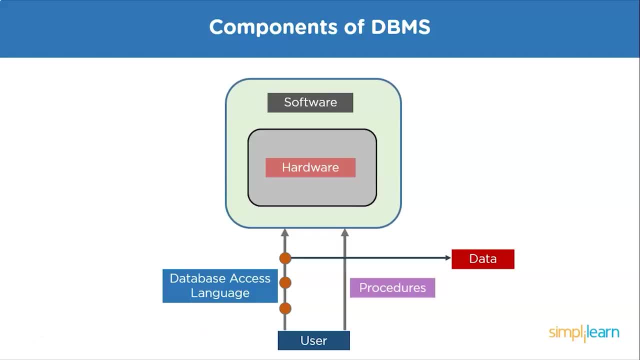 to form a database management system. and let's dive into these components: hardware: when we say hardware we mean computer hard disk, input output channels for data and any other physical component involved before any data is successful in the database. When we run Oracle or MySQL on a personal computer, then the 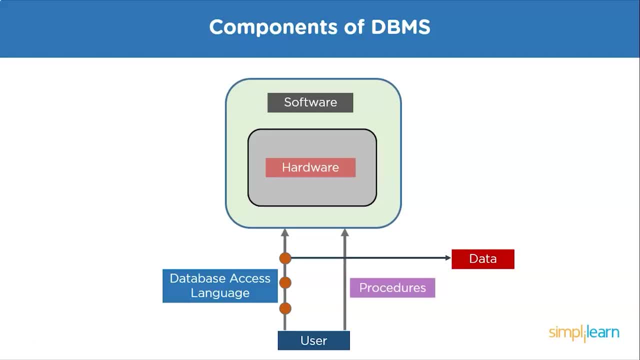 computer's hard disk, our keyboard using which we type in all the commands, our computers, RAM, ROM- all becomes a part of the DBMS hardware software. this is the main component, as this is the program which controls everything. the DBMS software is more like a wrapper around the physical database which provides us. 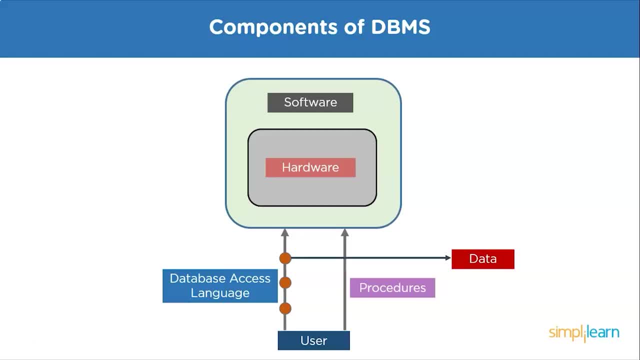 with an easy-to-use interface to store, access and update data. the DBMS software is capable of understanding the database access language and, interpreted into actual database commands, execute them on the database data data is that resource for which DBMS was designed. the motive behind the creation of DBMS was to store and utilize data in a typical database, the user save data if present, and METADATA put metadata. metadata is data is stored. Metadata is data is store by usingimerk s and errors. this khiano we said that we provide data. user has to do some demos before full session. is a database data? well, in this case that. 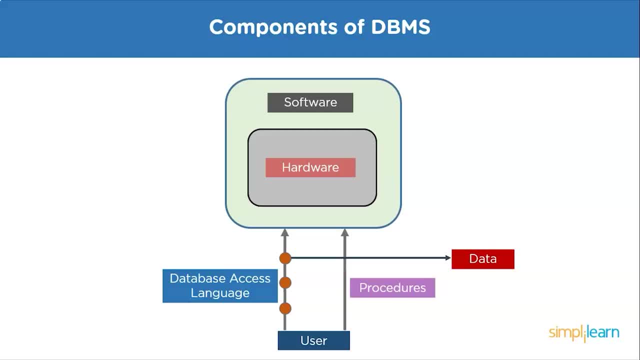 in settingños. we will create data over it about the data. this is information stored by the DBMS to better understand the data stored in it. for example, when I store my name in a database, the DBMS will store when the name was stored in the database. what is the size of the? 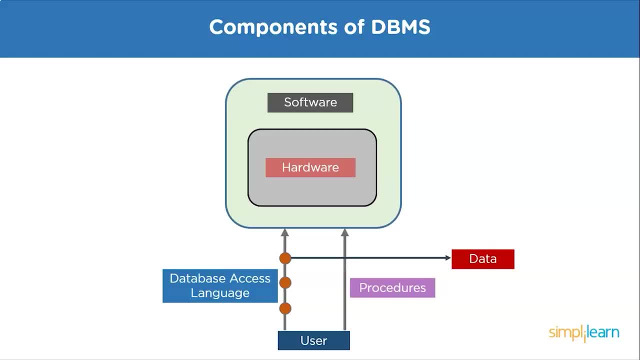 name. is it stored as related data to some other data or is it independent? all this information is metadata procedures. procedures refer to general instructions to use a database management system. this includes procedures to set up and install a DBMS, to log in and log out of DBMS software to manage databases, to 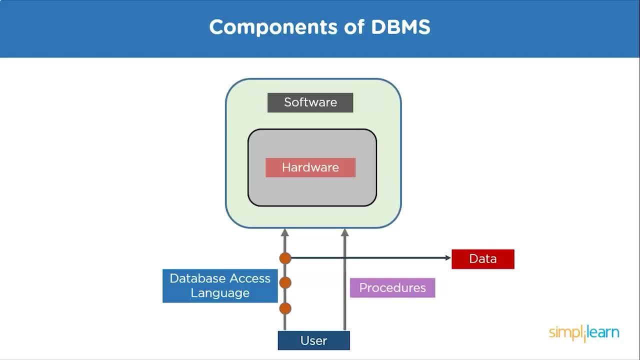 take backups, generating reports, etc. database access language. database access language is a simple language designed to write commands to access, insert, update and delete data stored in any database. a user can write commands in the database access language and submit it to DBMS, DBMS for execution, which is then translated and executed by DBMS. 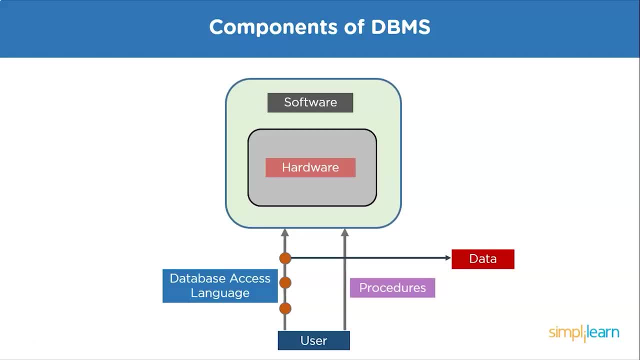 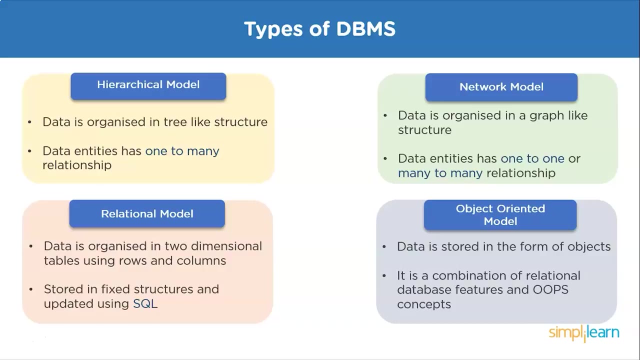 user. user can create new databases, tables, insert data, fetch stored data, update data and delete the data using the access language. now we'll see types of database management systems. we have quite many databases, but we will discuss few. first. is hierarchical model: this type of DBMS employees, the 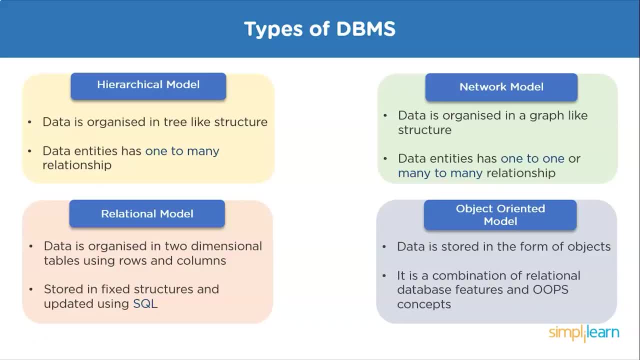 gonomon child relationship of storing data. Its structure is like a tree, with nodes representing records and branches representing fields. The Windows registry used in Windows XP is a hierarchical database, example Network model. This type of DBMS supports many-to-many relations. It usually results in complex database. 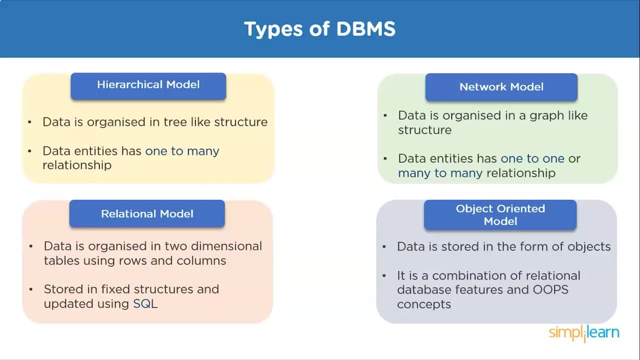 structures. RDMServer is an example of database management system that implements the network model- Relational model. This type of database defines database relationships in the form of tables. It is also called relational DBMS, which is the most popular DBMS type in the market Database. example of the 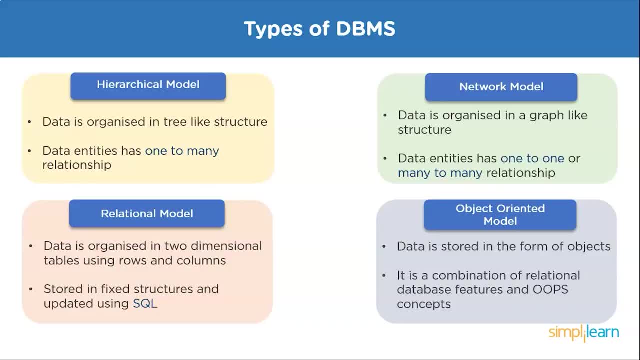 RDBMS system include MySQL, Oracle and Microsoft SQL Server database. Object-oriented model: This type of computer's database supports the storage of all data types. The data is stored in the form of objects. The objects to be held in the database have attributes and 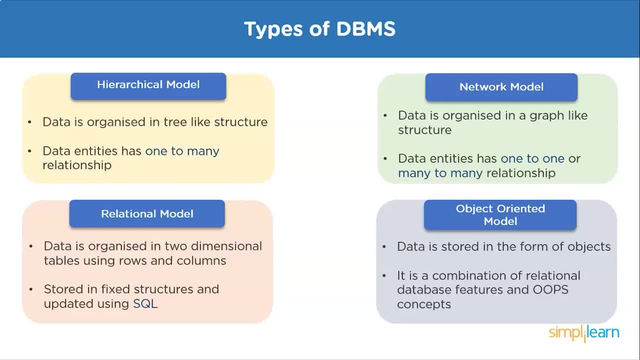 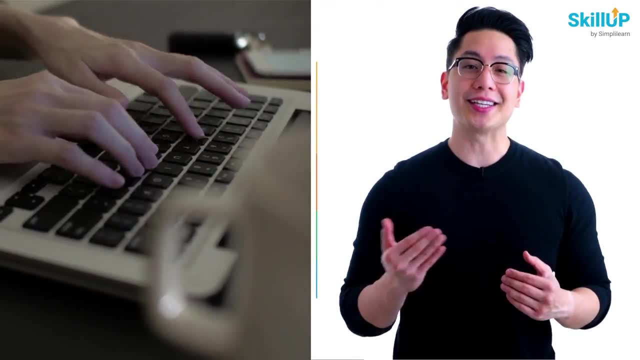 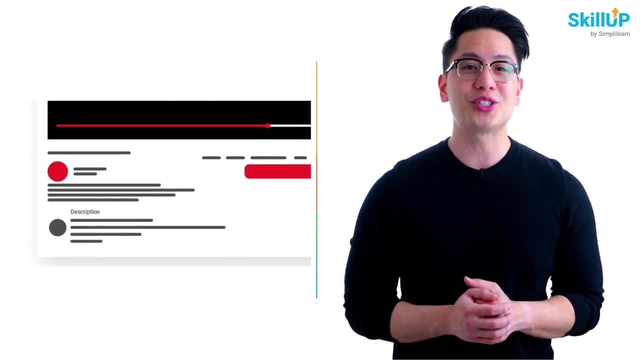 methods that define what to do with the data. PostgreSQL is an example of an object-oriented relational DBMS. If getting your learning started is half the battle, what if you could do that for free? Visit SkillUp by SimplyLearn. Click on the link in the description to know more. 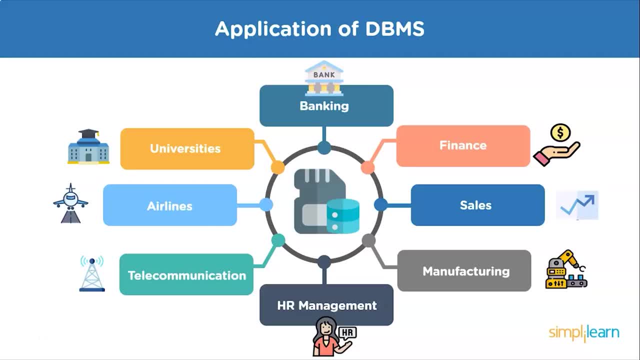 Now we come to the applications of DBMS. There are different industries having the application of DBMS. Like telecom industry, There is a database to keep track of the information regarding calls made, network usage, customer details, etc. Without the database systems it is hard to maintain that huge. 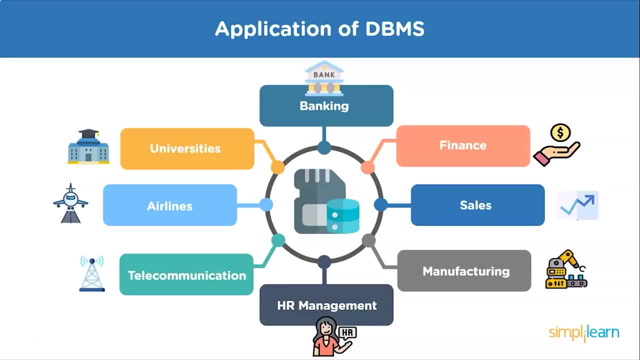 amount of data that keeps updating every millisecond. Manufacturing industry, Where it is a manufacturing unit, warehouse or distribution center, Each one needs a database to keep the records of the data. There are many other applications, like in and outs, For example. distribution center should keep a track of the product. 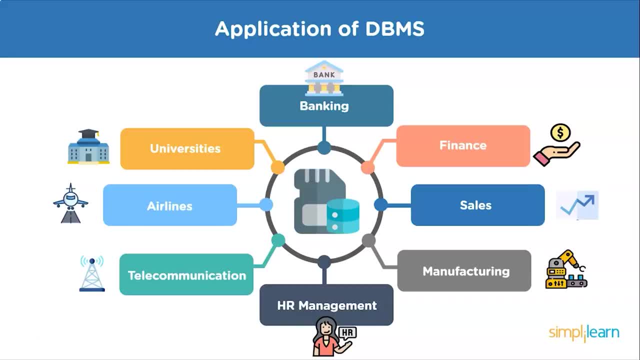 units that supplied into the center, as well as the products that got delivered out from the distribution center on each day. This is where DBMS comes into picture: Banking system For storing customer info, tracking day-to-day credit and debit transactions, generating bank statements, etc. All this work has been 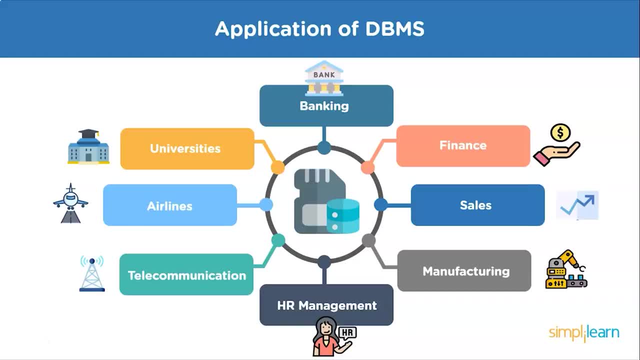 done with the help of database management Sales To store customer information, product information and invoice details. Airlines To travel: through airlines we make early reservations. This reservation information, along with flight schedule, is stored in database. Education sector Database systems are frequently used in schools and colleges to store and. 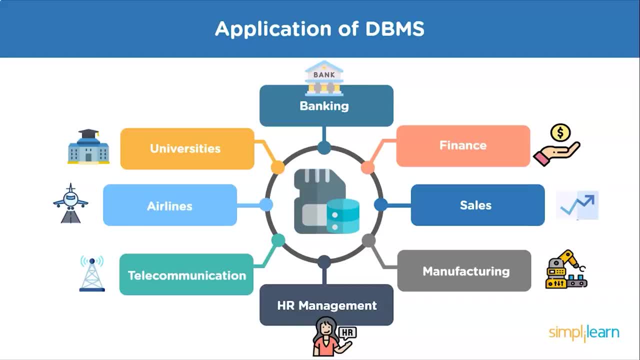 retrieve the data regarding student details, staff details, course details, exams details, payroll data, attendance details, fee details, etc. This is a hell lot amount of interrelated data that needs to be stored and retrieved in an efficient manner. Online shopping: You must be aware of the online shopping websites, such as Amazon, Flipkart. 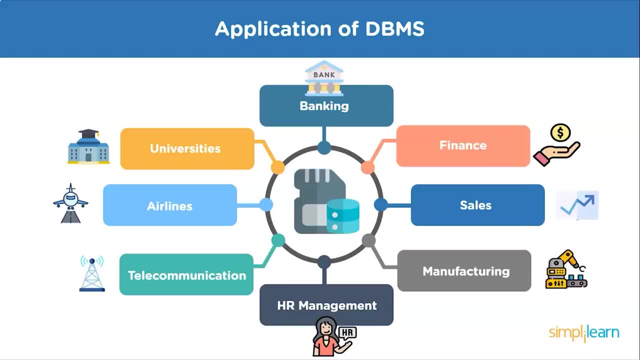 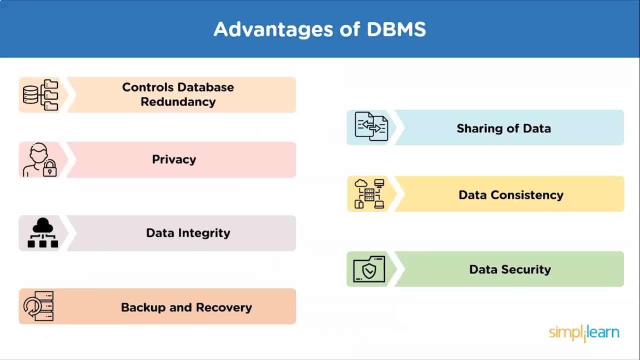 etc. These sites store the product information, your addresses and preferences, credit details and provide you the relevant list of products based on your query. All this involves a database management system. Compared to the flat file system data, the database management system has many advantages. 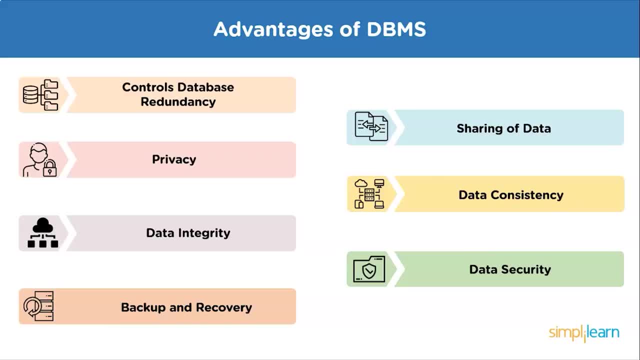 Some of these advantages are: Reducing data redundancy. The file-based data management systems contain multiple files that were stored in many different locations in a system or even across multiple systems. Because of this, there were sometimes multiple copies of the same file, which lead to data. 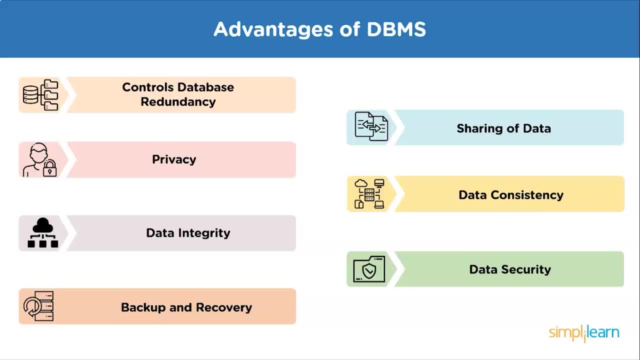 redundancy. This is prevented in a database, as there is a single database and any change in it is reflected immediately. Because of this, there is no chance of encountering duplicate data. Sharing of data In a database: the users of the database can share the data among themselves. 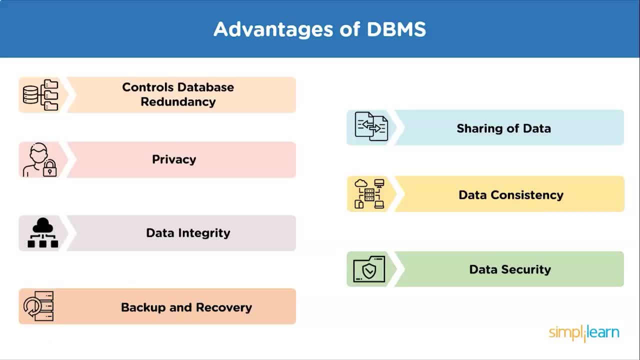 There are various levels of authorization to access the data and, consequently, the data can only be shared based on the correct authorization protocols being followed. Many remote school users can access the database simultaneously and share the data between themselves. Data Integrity: Data integrity means that the data is accurate and consistent in the 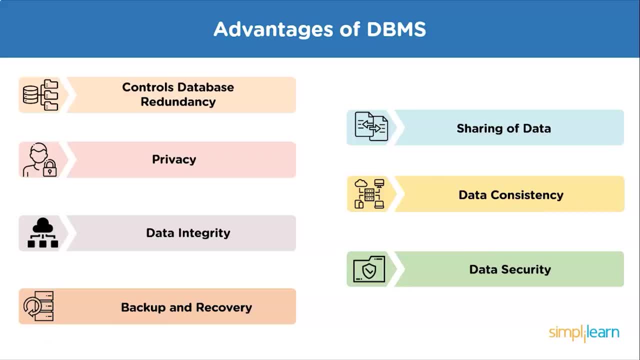 database. Data integrity is very important, as there are multiples databases in a DBMS, So it is necessary to ensure that the data is correct and consistent in all the databases and for all the users. Data security: Data security is a vital concept in a database. 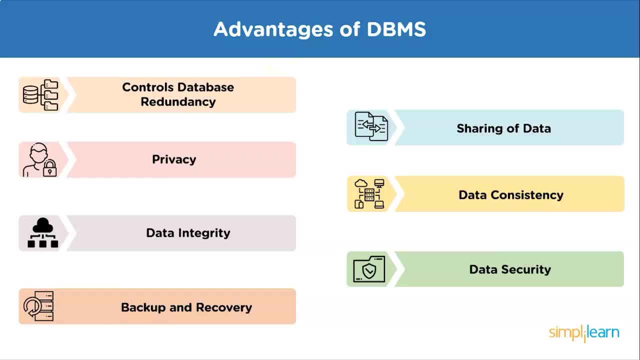 Which means data integration means that all the databases in a database work under one rióuct. In my previous video I explained the nature and similarity between other main a database. only authorized users should be allowed to access the database and their identity should be authenticated using a username and password. unauthorized users should not be allowed to. 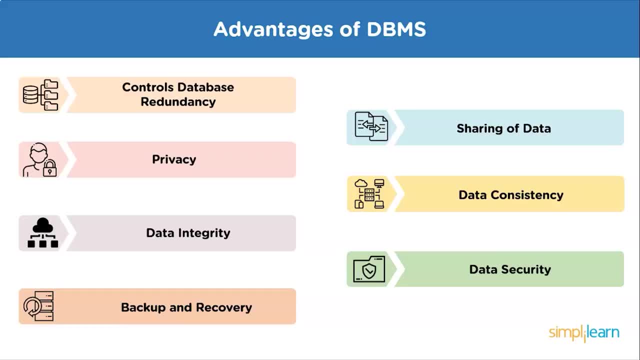 access the database under any circumstances, as it violates the integrity constraints. privacy: the privacy rule in a database means only the authorized users can access a database according to its privacy constraints. there are levels of database access and a user can only view the data he is allowed to, for example, in social networking sites. access constraints: 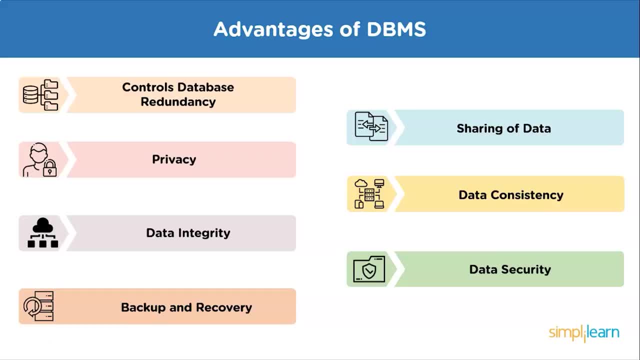 are different for different accounts. a user may want to access backup and recovery. database management system automatically takes care of backup and recovery. the users don't need to backup data periodically because this is taken care of by the dbms. moreover, it also restores the database after a crash or system failure to its previous condition: data consistency data. 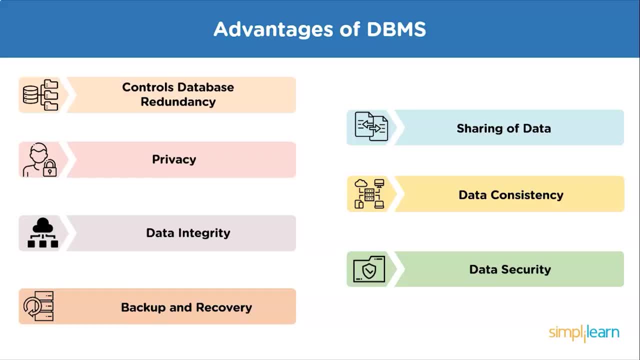 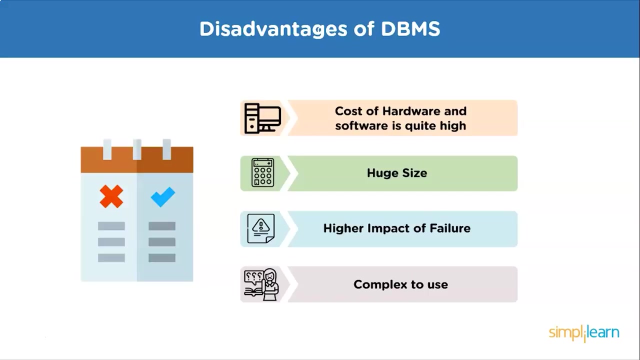 consistency is ensured in a database because there is no data redundancy. all data appears consistently across the database and the data is the same for all the users viewing the database. moreover, any changes made to the database are immediately reflected to all the users and there is no data inconsistency. now we see what are the disadvantages of tbms. first is high cost- the high